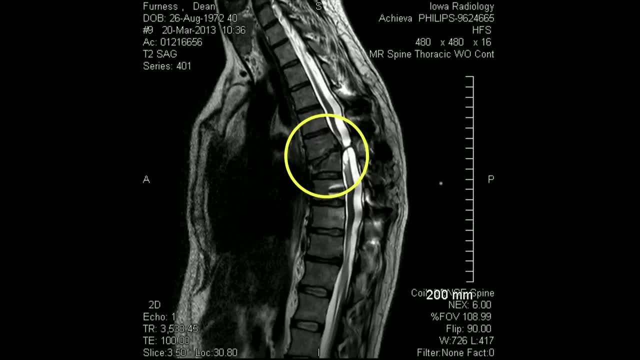 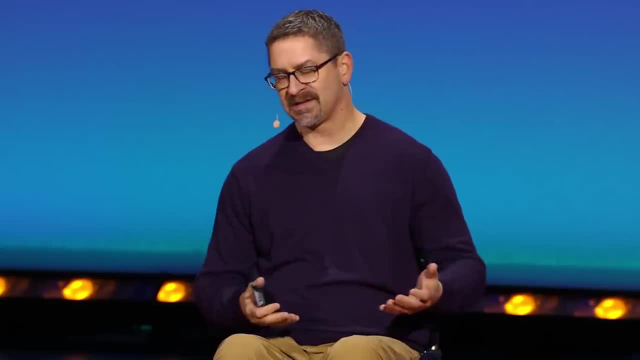 And in the process I was told I'd probably never walk again. It became very normal for me to use a rope to sit up in bed because my abdominal muscles no longer work, or to use a board to slide out of bed into a wheelchair. 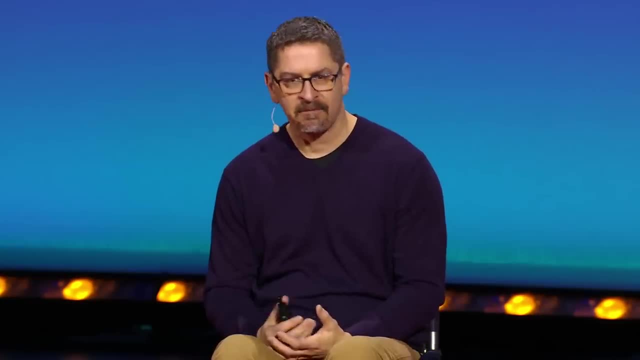 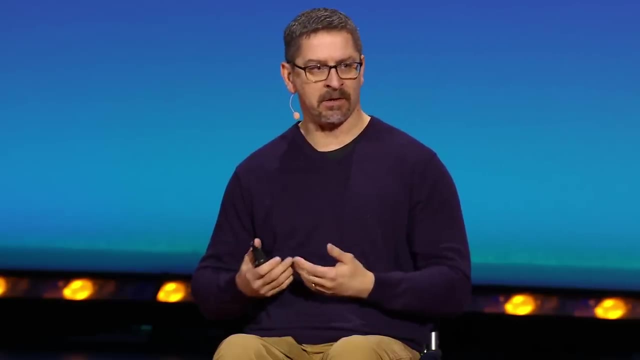 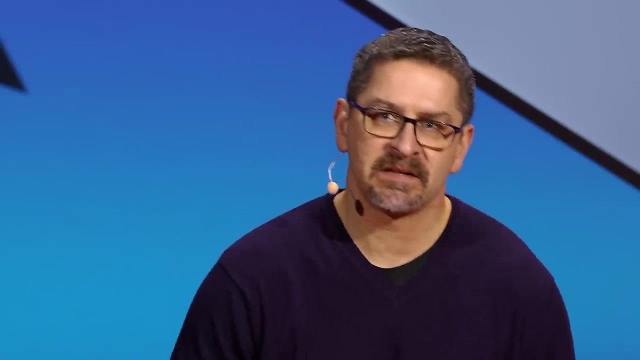 or to even wait for people to reach things for me. Everything that I had learned and had known about my height and my strength and my balance and my mobility was blown away. My entire personal average had been reset. Now, you can be sure, in those days, 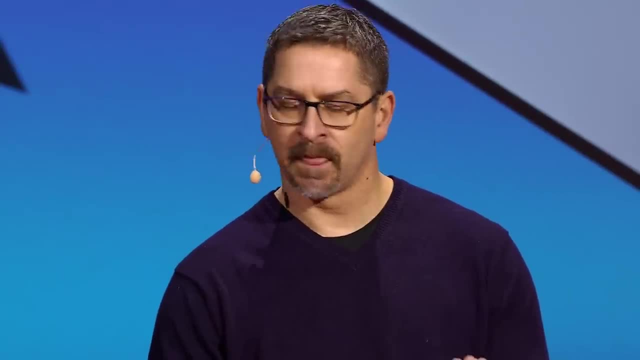 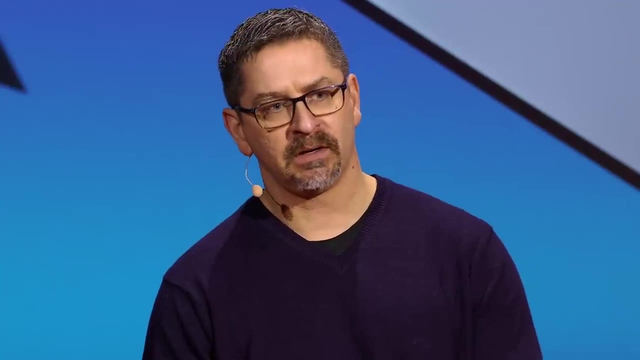 I was being measured more than ever, by the doctors and nurses for sure, but maybe more so in my own mind, And I found myself comparing what I thought I was going to be able to do going forward with what I once was able to do. 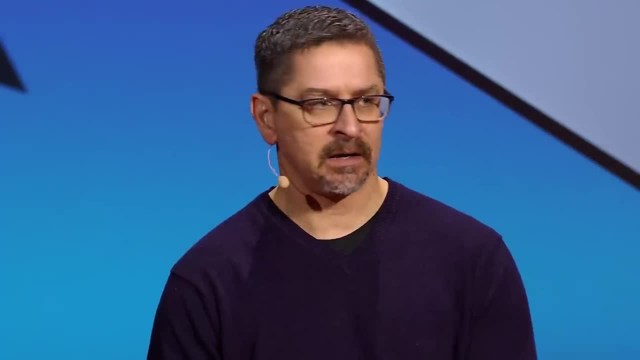 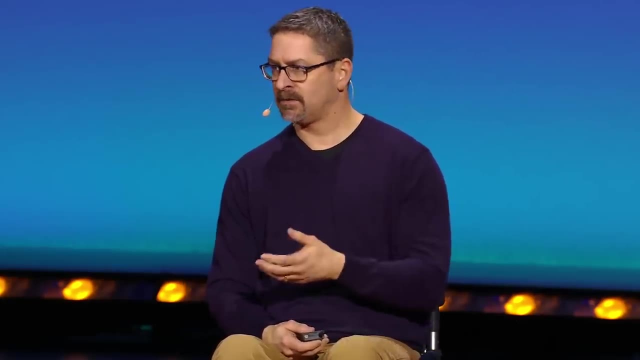 And I became pretty frustrated. It took some very consistent prodding from my wife who kept saying: get your eyes up before I could get moving forward, And I soon realized that I almost had to forget about the person I was before and the things I was able to do before. 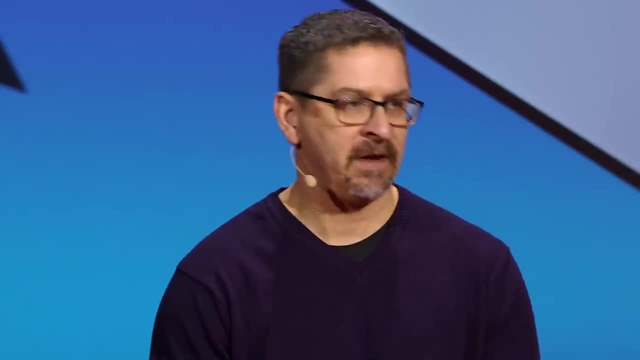 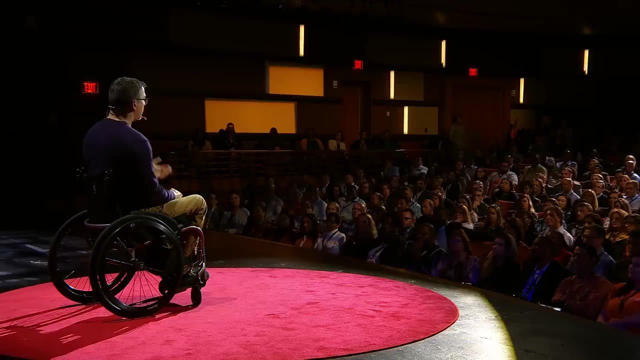 I almost had to pretend it was never me, And I'm afraid, if I had not made that realization, my frustration would have turned into something much harder to recover from Now. luckily, a few weeks later I was transferred to a specialty spinal cord rehab hospital. 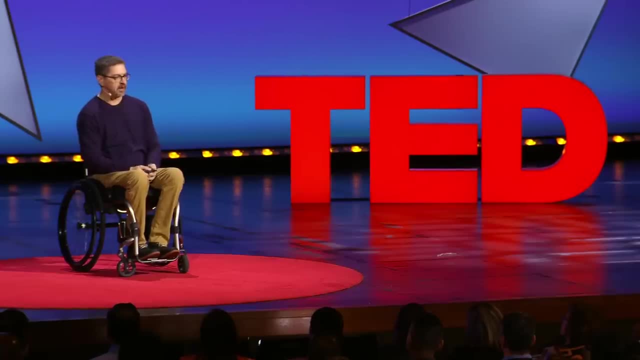 about 10 hours from home And wouldn't you know, the first day of rehab and the first session, we had something called fit class And a group of us broke into teams to see which team could do the most reps in the weight machine. 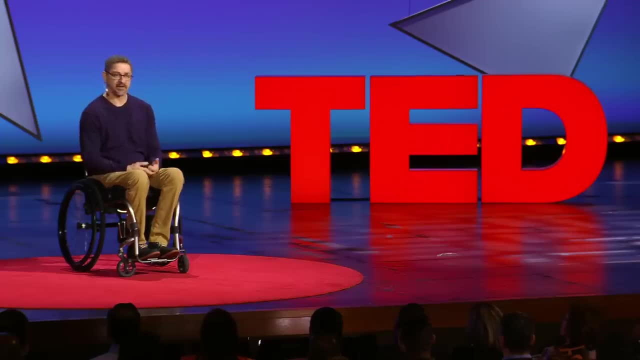 Now we've all been there, haven't been to the gym in a year or two, and neither had I, And so what do you do? You try to do what you did a couple of years ago: You do a couple of sets. 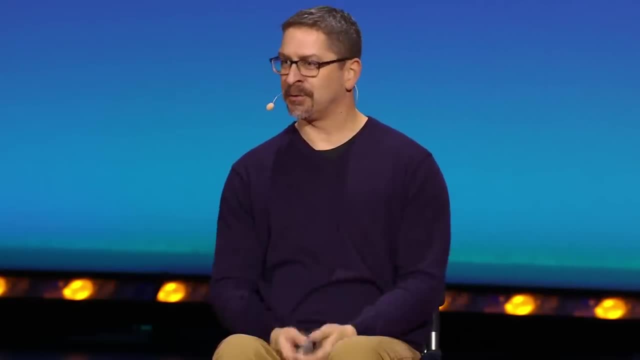 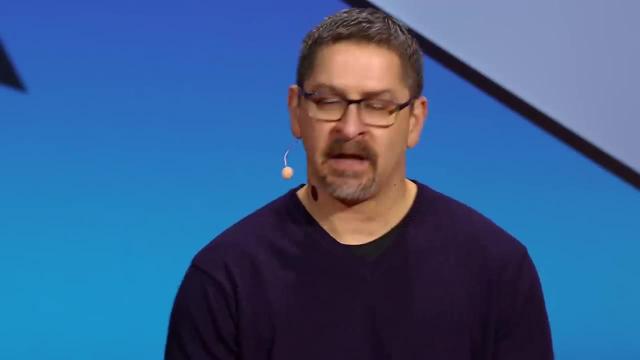 And then what do you do? A couple more And you're feeling even better. so you do more, And the next two weeks you complain to your family about how sore you are. Well, my team went all out and we won. 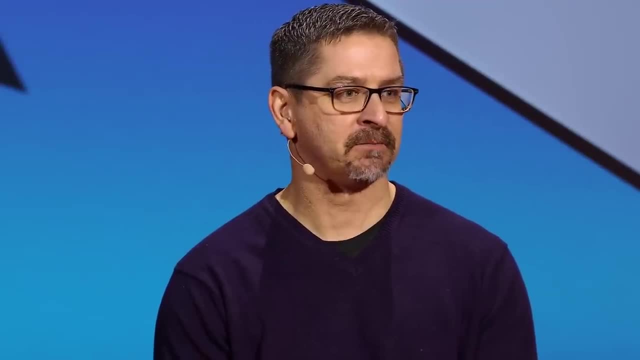 We won big, We won big, And from the next three days I could not straighten my arms, Which isn't that big a deal, except when you're in a wheelchair, And that's really what you have to use to get around. 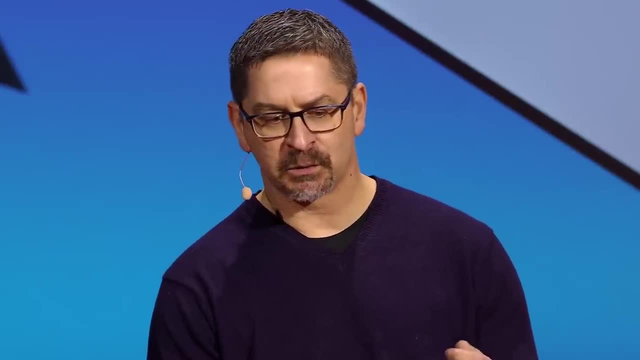 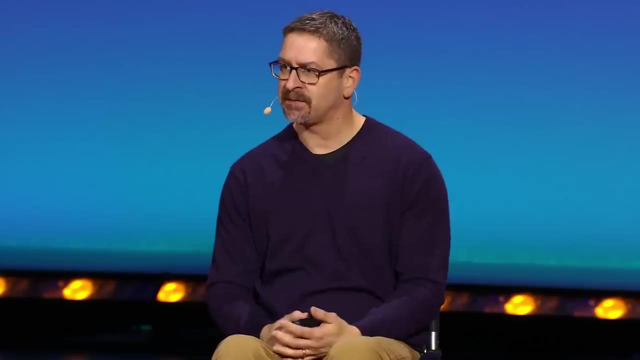 And that proved to be a very important lesson for me. You know, it was one thing that I couldn't compare myself to myself. but even around people in the same situation in that hospital, I found that I couldn't try to keep pace or set pace with them as well. 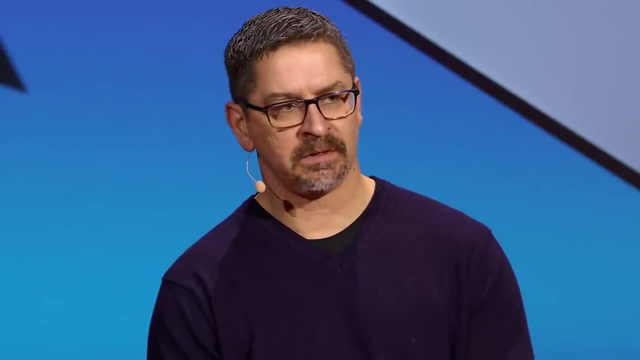 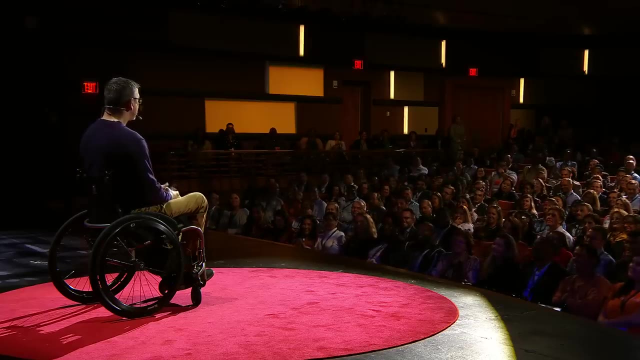 And I was left with really only one choice, and that was to focus on who I was at that point in time, with where I needed to go, and to get back to who I needed to be For the next six weeks, for seven to eight hours a day. 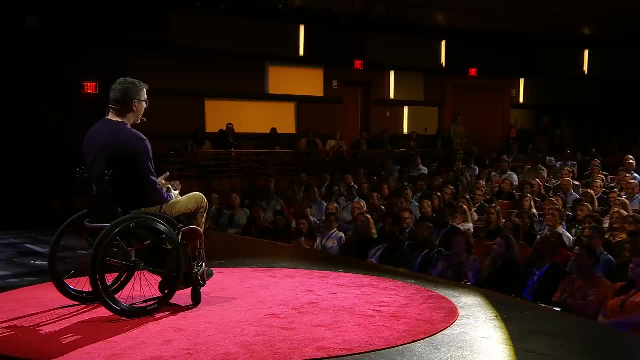 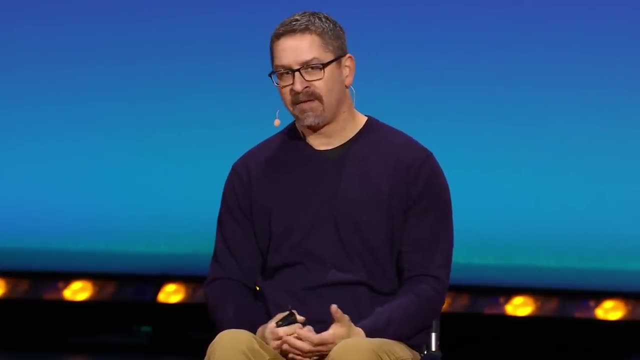 that's what I did. I built little by little And, as you might expect, when you're recovering from a spinal cord injury, you're going to have a bad day. You might have a few in a row, And what I found out is that good and bad. 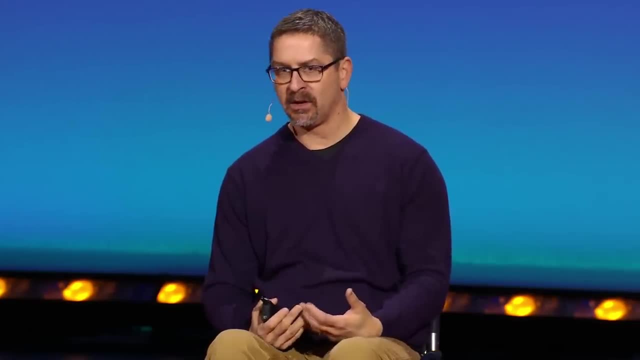 really didn't have a lot of meaning unless I had the context of knowing what my average was. It was really up to me to decide if something was bad or good based on where I was at that point in time, And it was in my control to determine. 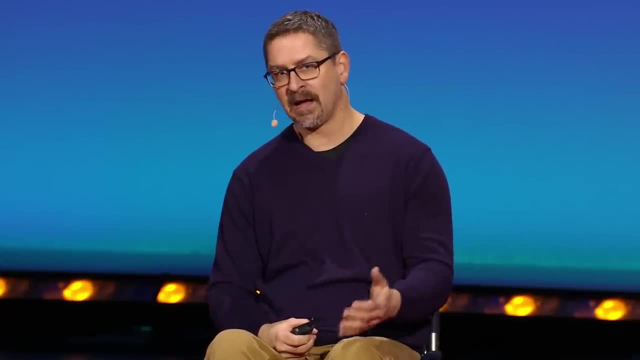 if it really was bad or good, And it was in my control to determine if it really was a bad day. In fact, it was my decision on whether or not I could stop a streak of bad days And what I found during that time away from home. 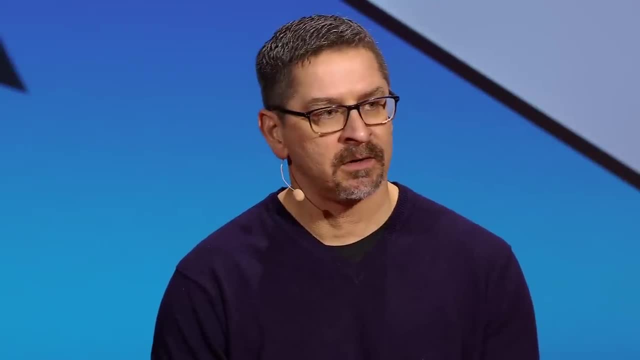 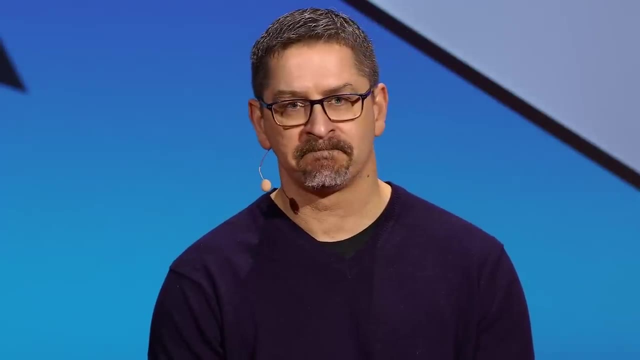 is, I never had a bad day, even with everything going on. There were parts of my day that were certainly not as pleasant as they could be, But it was never an entirely bad day. So I'm guessing all of you have been through a meeting. 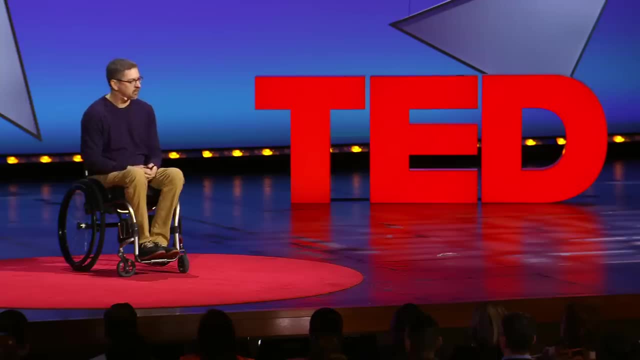 that probably didn't go very well, or a commute that wasn't as great as you would like it, or even burned dinner at night. Did those things really ruin your entire day? What I've found in those scenarios is the quicker you move on to what's next. 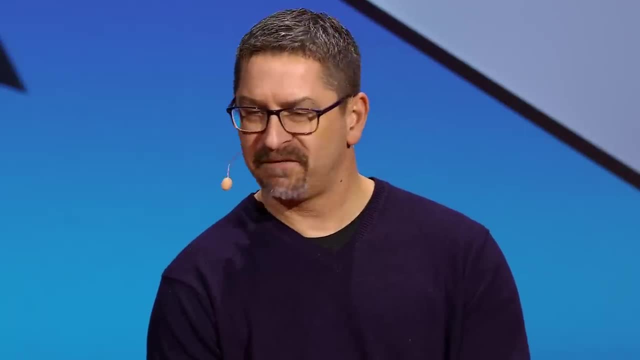 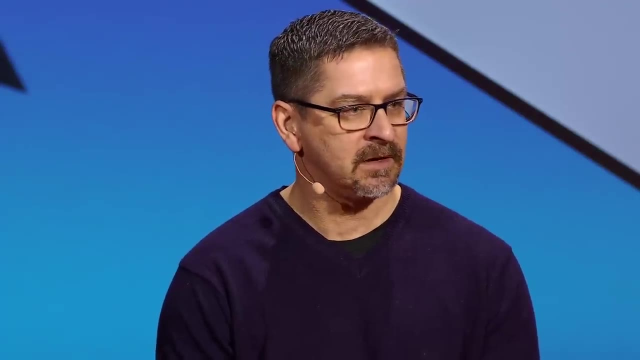 the quicker you can start attacking things And by moving on to next as fast as possible, you shrink the time you spend in those bad scenarios and it gives more time for the good And, as a result, the good outweighs the bad. 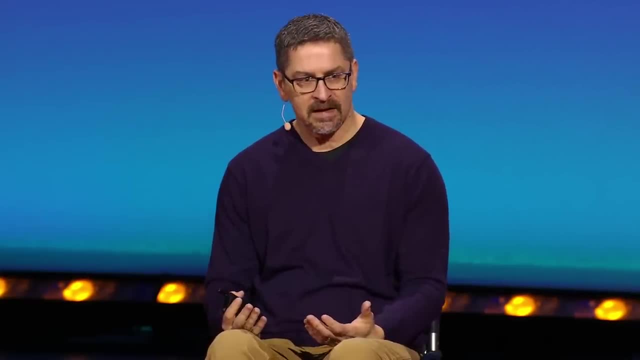 your average increases, and that's just how the math works. It didn't matter to me if I had spent the morning really struggling with my medication, or at lunch, my legs being very spastic, or even if I had fallen out of my wheelchair. 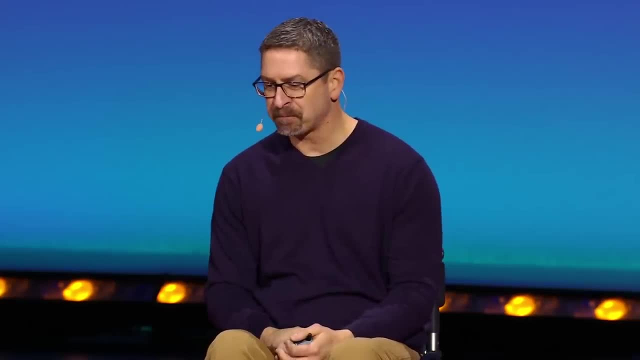 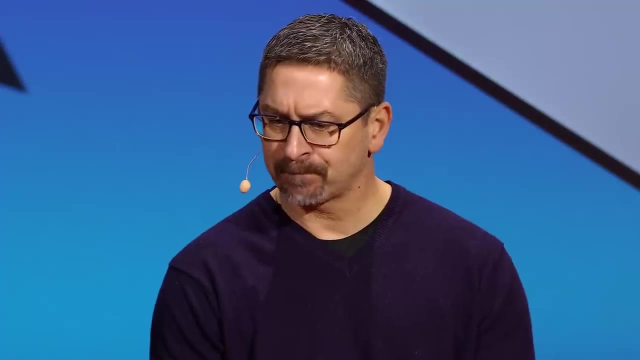 Ask my wife. it happens quite often She's here. There were just small parts of my day and small parts of my average, And so in the months and years that followed, I continued to try to attack things in that way And, before I know it, 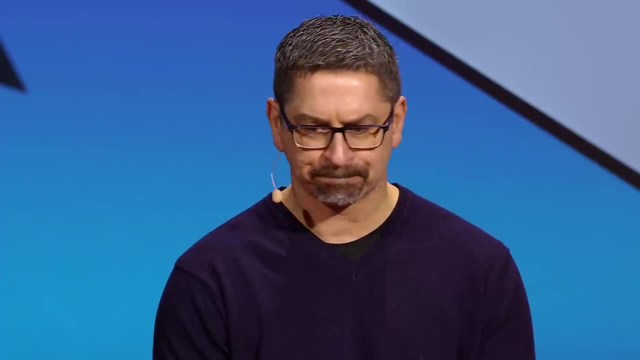 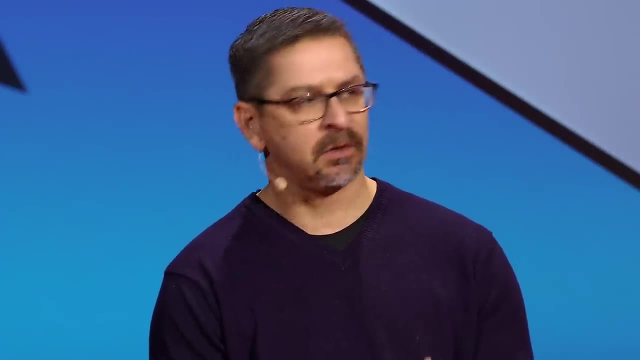 I was being presented with some pretty incredible challenges, like completing a marathon in a wheelchair In early 2016,. I met my physical therapist and after a few really grueling sessions, she must have sensed something, because she pulled me aside and said: 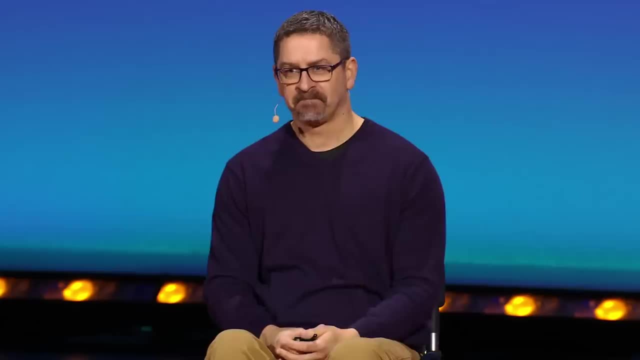 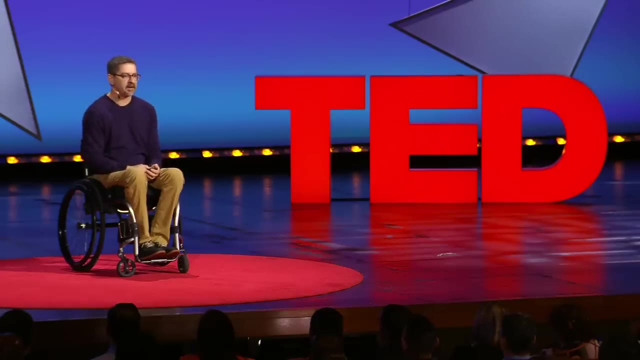 you know you should do a half marathon In your wheelchair. Oh yeah, it's in 10 weeks. And I thought in my mind: you're crazy. I didn't have a workout plan. I didn't have any way of knowing how fast I needed to go. 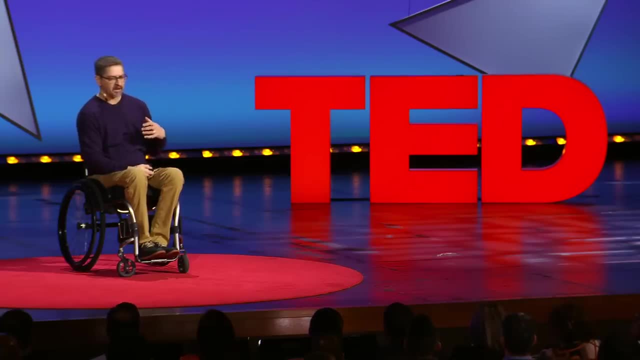 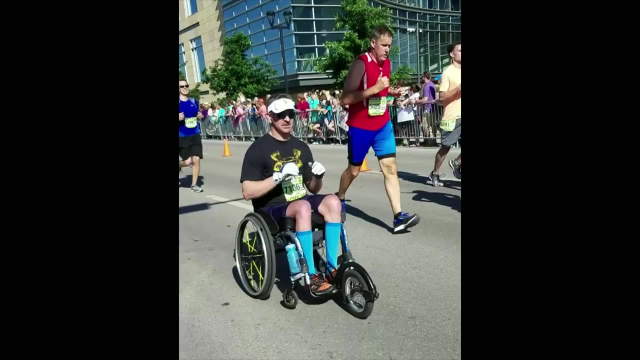 or how far I was supposed to go. But I simply got to work And I started tracking every workout every day and I simply wanted to be as good as or as fast as I was the prior day And in the end I really created that average for myself. 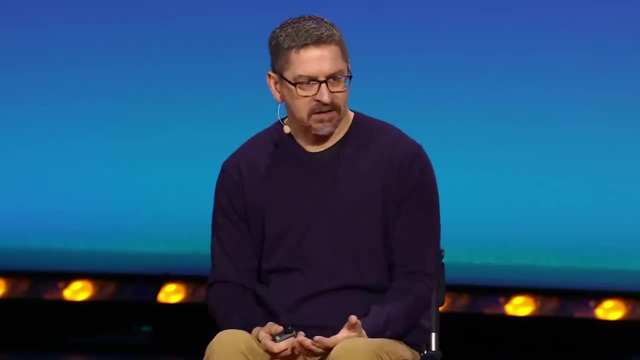 and I tried to build on that as much as I could. Well, I finished that race right in time with what my average should have been, And you know, somewhere along the way I kind of closed the door on who I once was. 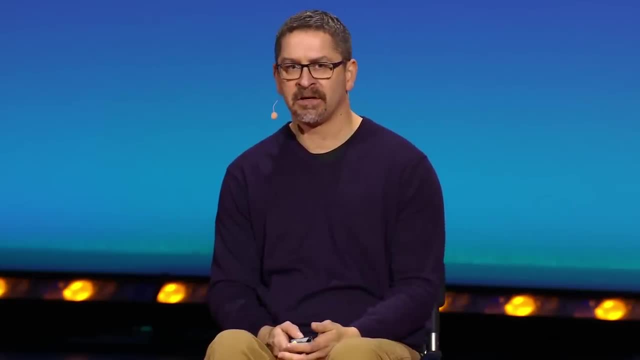 That person, who I was before and all those things I thought I was able to do. it really didn't matter. In fact, walking again really didn't matter. It became much less of a goal for me in terms of where I was going to go. 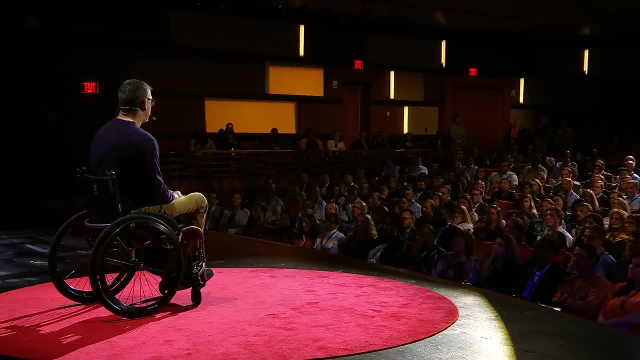 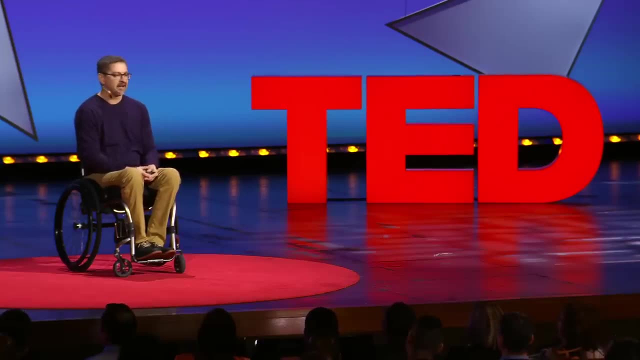 And besides, you guys are so slow when you walk- I mean, in crowds like this, it is so difficult. I'm like get out of the way. We're going places And all I wanted to do was go fast. So I did what I thought I should do. 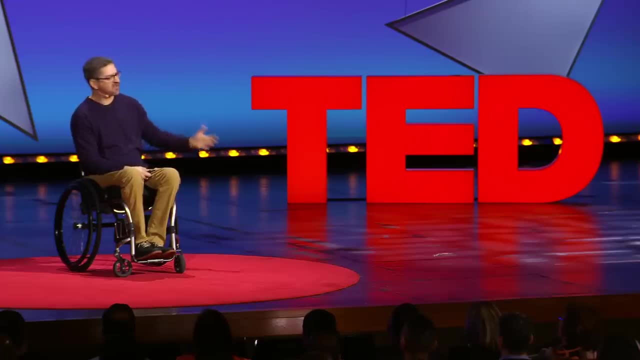 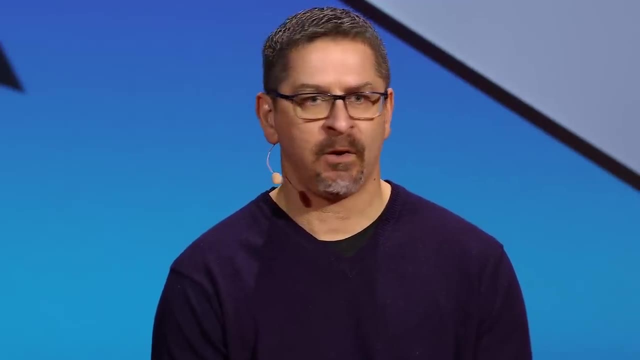 I started researching wheelchair racing And I went online and I found the best of the best. I learned their technique, I learned about the equipment And I was lucky to have a coach that offered me a way to get started. And after talking with him, 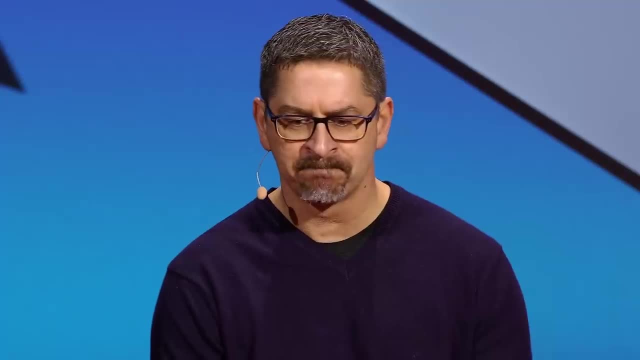 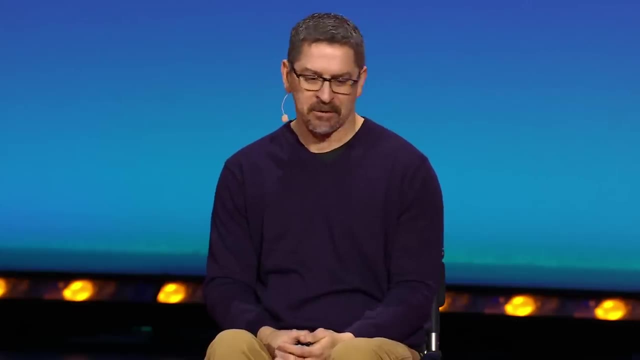 and having him help me get those things underway. I was like, as I was leaving, he says: you know you should do the 2017 Chicago Marathon And you know he's the coach. I can't tell him no. 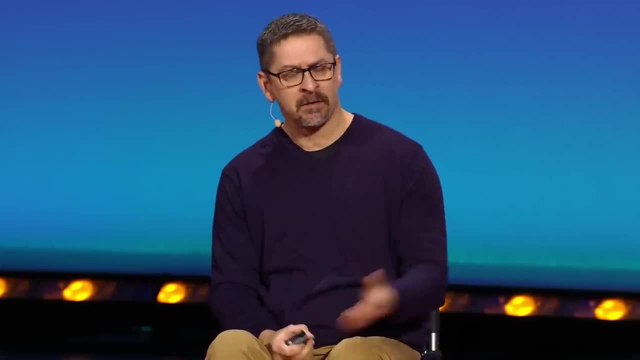 So with that guidance I went back home and I got to work much like in the prior way And I continued researching. but I had learned my lesson. I was really careful not to compare with how accomplished those people on the Internet were and how fast they were. 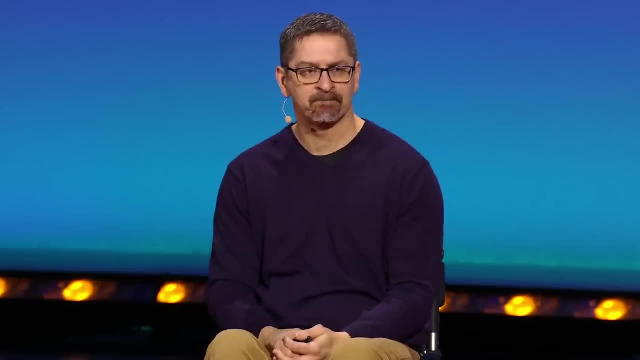 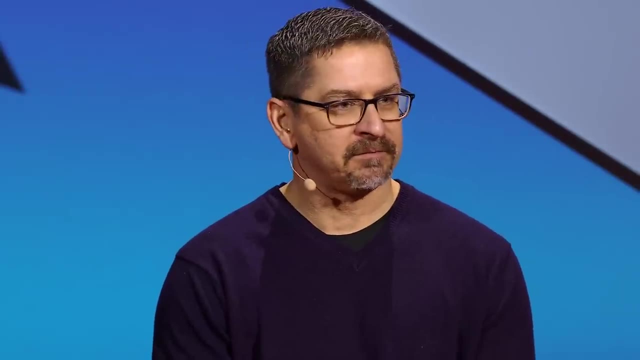 because if I had, then I probably never would have continued going through with it. Well, the weekend of the race arrived and it was just like going to college. It was just like going to college for the first time: You're dumped off. 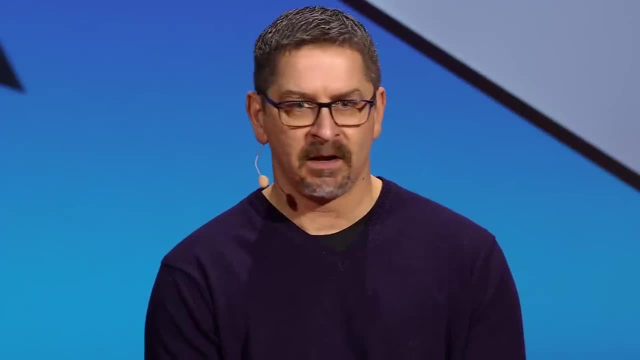 There's a whole bunch of people around you. You don't really know very many of them. Somebody's got the cool stereo and the cool TV and they're smart and they're pretty and they're cute and they're handsome. 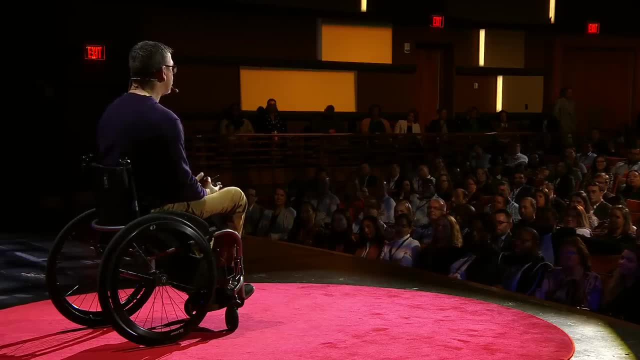 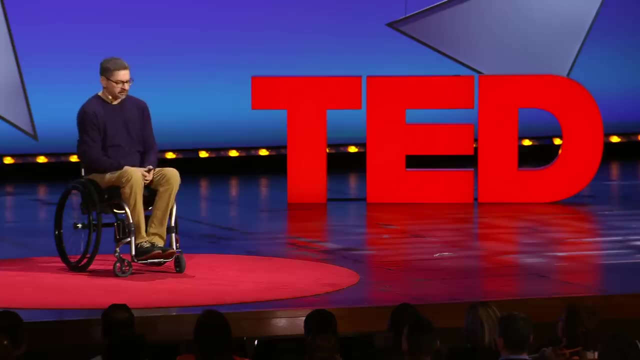 and you don't know if you really belong. But then somebody says, hey, let's go get food. And all of a sudden that friend group happens and you start to settle in. Well, that weekend of the race we had a meeting called the Wheelers' Meeting. 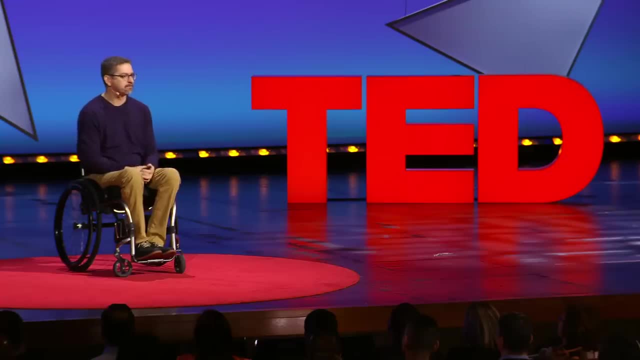 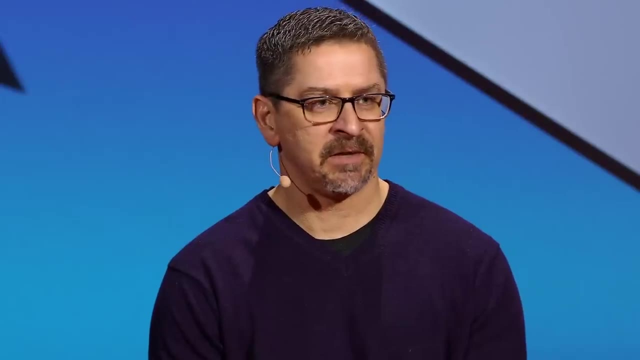 and there were 60 wheelchairs in that room the night before the race And I was like, wouldn't you know it? all of the people that I had been researching were there- the best in the world. There must have been over 50 Paralympic medals in the room that day. 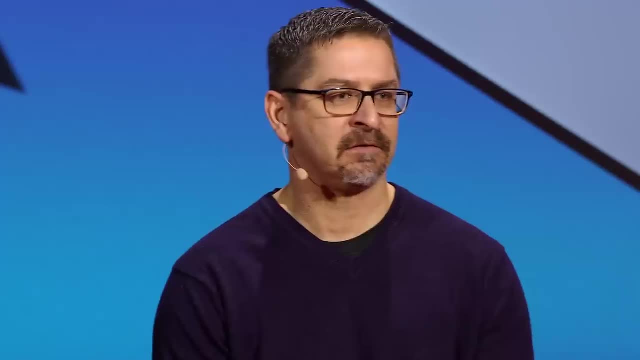 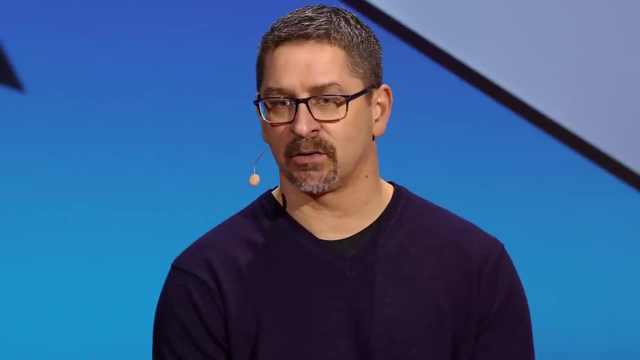 And I felt pretty small and I fell back into that trap of comparing myself. I knew that my averages that I had been tracking during my workouts- were over 90 seconds slower per mile than theirs, And the coach was the only one there that I knew. 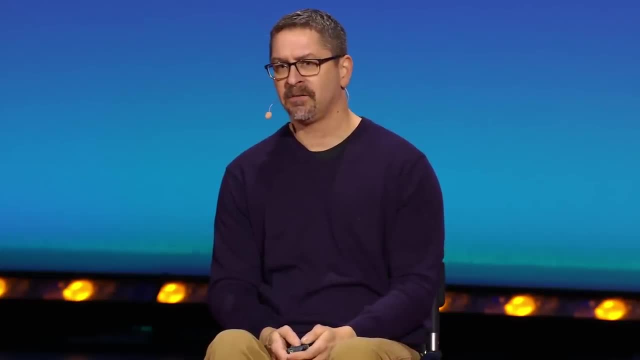 and he reached out and noticed something and I think he sensed my anxiety and he invited me to get food with his team And with that everything settled down. I realized really quick that they didn't care about my average, surely, and I had forgotten about theirs. 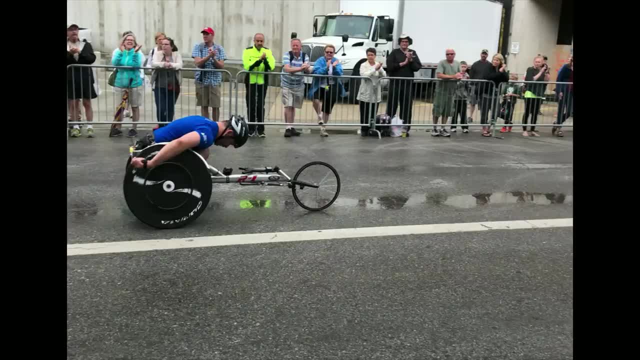 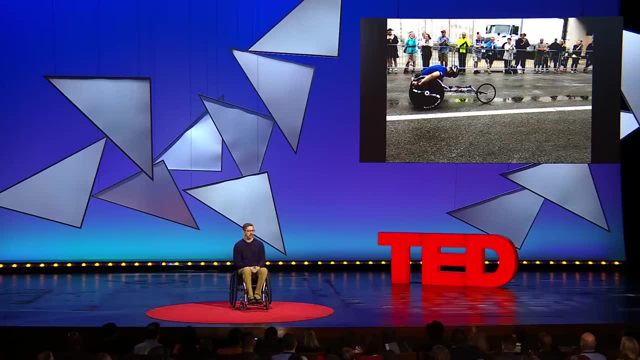 Well, that next day I finished the race about 45 minutes after the person that won it. But as I was leaving, those new friends who are very close today, challenged me to stay involved and to keep working through different races and competitions, And so I did what I knew how. 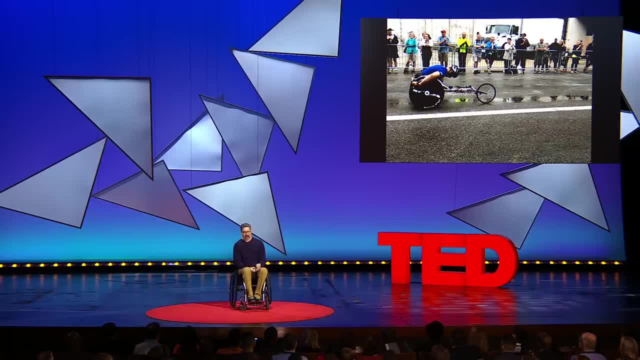 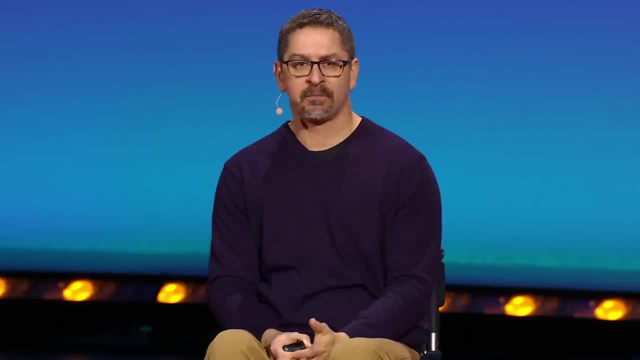 I went home and I got busy. Now, as you can imagine, being in a wheelchair, let alone training for a marathon in a wheelchair, is a pretty lonely thing. I have an incredible group of friends that will ride bike with me and keep track of pace and help me out. 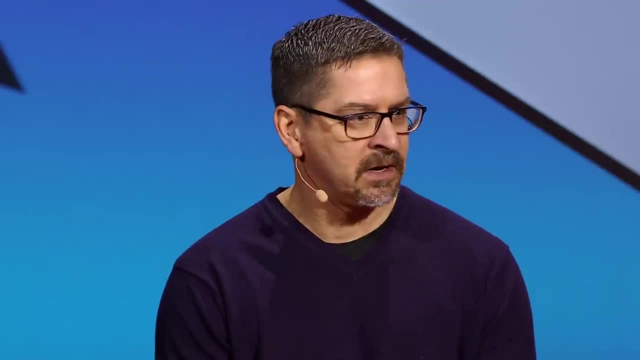 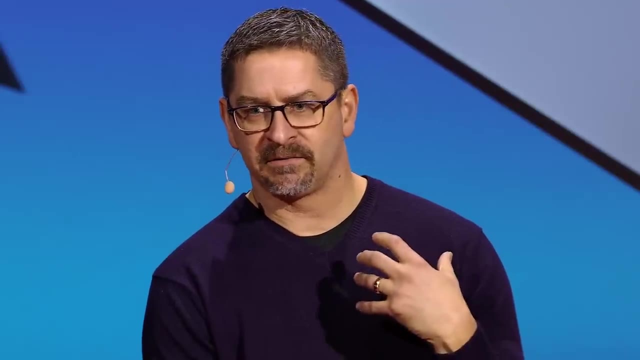 But in the end it's still five to six days a week, it's 50 to 60 miles of effort and it's a lot of alone time And for the most part you really have nothing to rely on but yourself in those times. 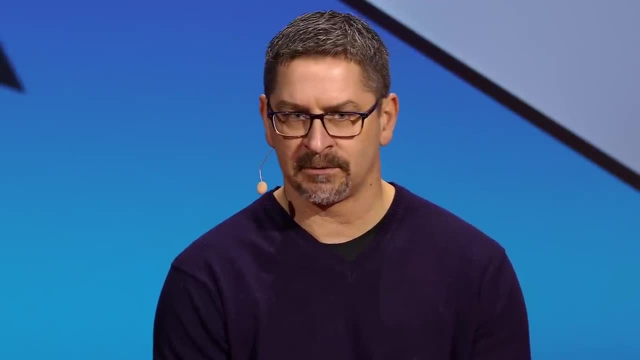 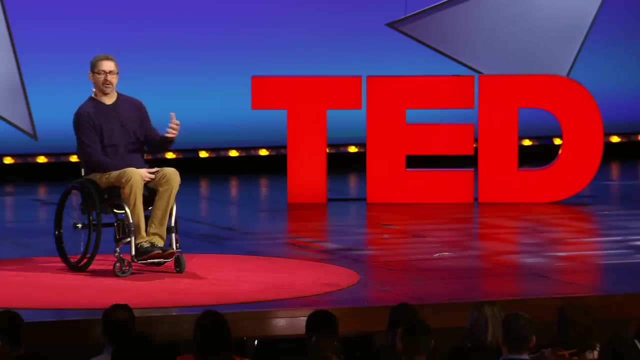 It's my average and I'm trying to get better little by little. Well, this fall I was in Chicago for the third time. It was my seventh marathon And, just like going back to college for your junior year, you're anticipating catching up with friends.